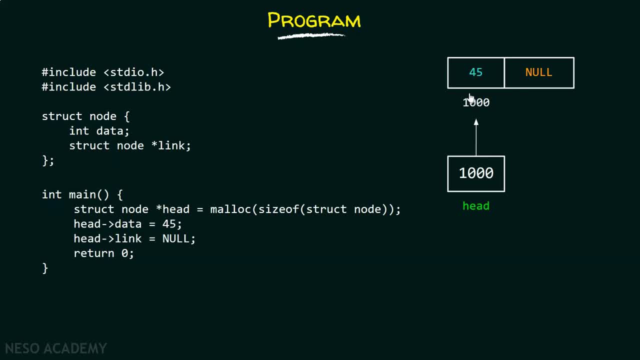 Now here is the head pointer which is pointing to the first node of the list. This is clear from this fact that, after allocating the memory, the address which is returned by this malloc will be the address of this node, that is, 1000.. This address will get stored within this head pointer. 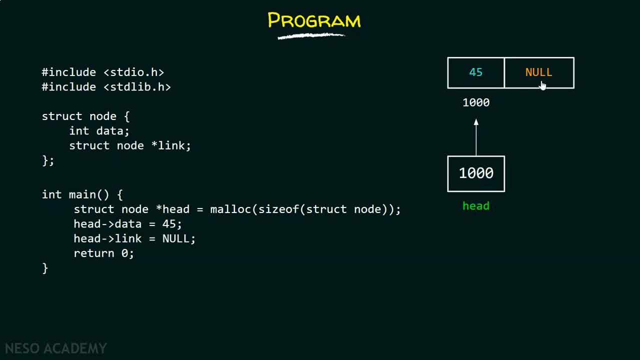 Now this head pointer can access data as well as the link part of this node, And that is what is done over here. The head pointer is accessing the data, and here I am trying to assign this value, 45, to it, And here in the link part, I am trying to assign null. 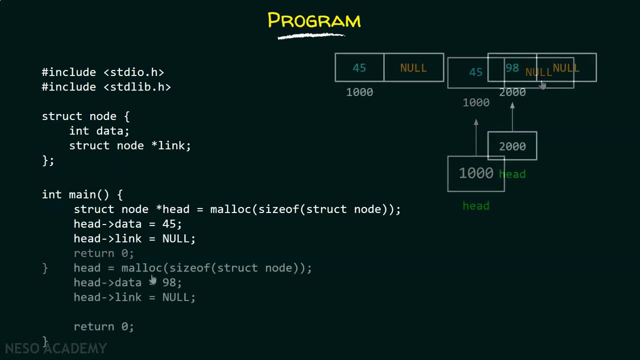 Initially it contains null. Later on it will get updated. Obviously, if we want to create the second node, we will again have to call this malloc function And then after that, here what I am doing: I am putting the address returned by the malloc into this head pointer. 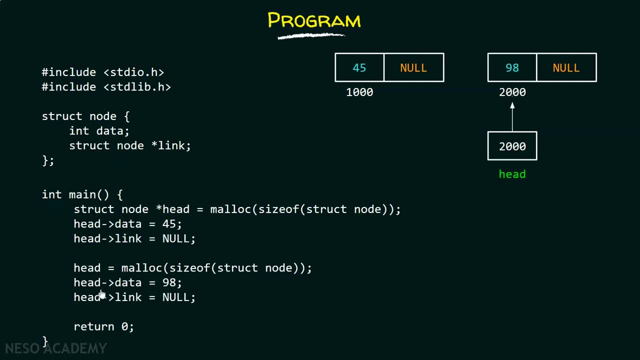 Now head is pointing to the second node of the list And obviously with the help of head pointer I am trying to assign 98 to data and null to the link part. But let me tell you there is some problem with this code. You can easily identify the problem as well. 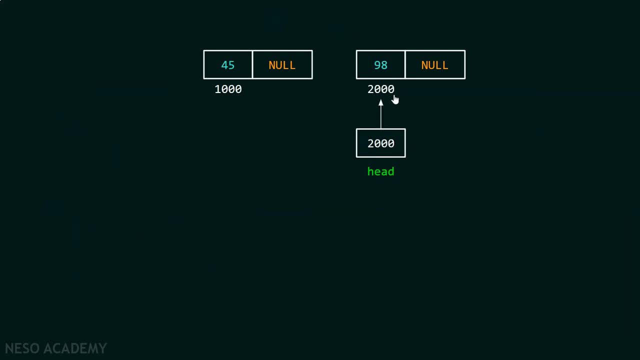 Basically, you can see that head pointer is pointing to the second node of the list, Isn't that? so Head is now pointing to the second node. Now there is no way to access the first node of the list. We have lost the reference of the first node. 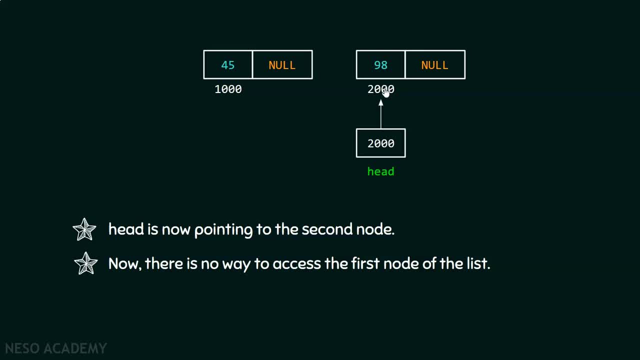 Previously, head was pointing to the first node, Now it is pointing to the second node. Now there is no way to access the first node of the list, Or there is no way to access this node at all. right, Because the only way to access this node is through this pointer. 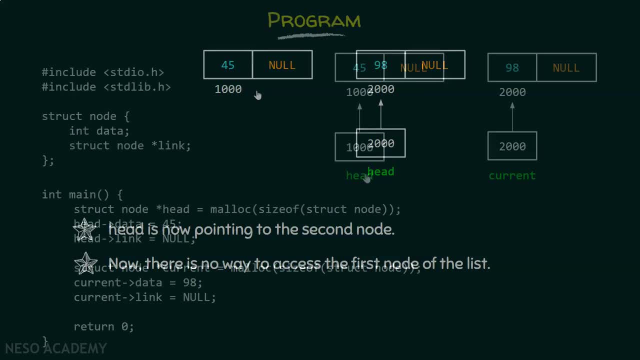 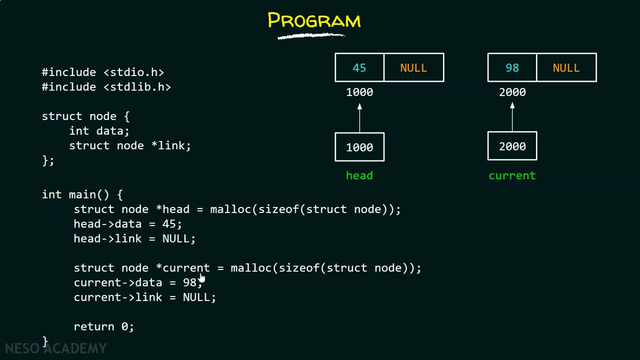 Now it is pointing to the second node. So what is the solution Here? we will create another pointer which will point to the second node Here. we will change this to current instead of head, And then now this current pointer is pointing to the second node of the list. 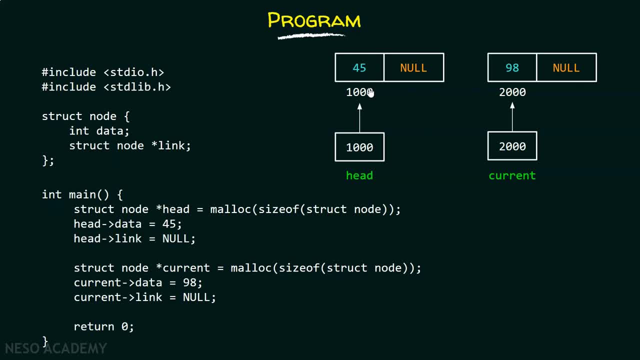 Head pointer is still pointing to the first node. Now, this is fine, because we haven't lost the reference of the first node at all. Head is still pointing to the first node And there is another pointer current which is pointing to the second node. 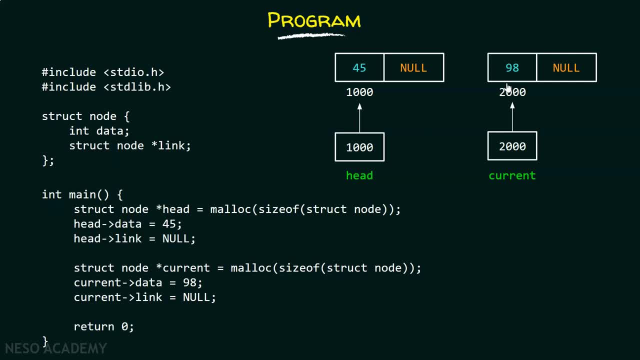 So everything is fine up to this point. Now the next step is to update the link part of the first node so that it can point to the second node. So here, this is the way we update the link part of the first node. The link part of the first node now contains the address 2000..